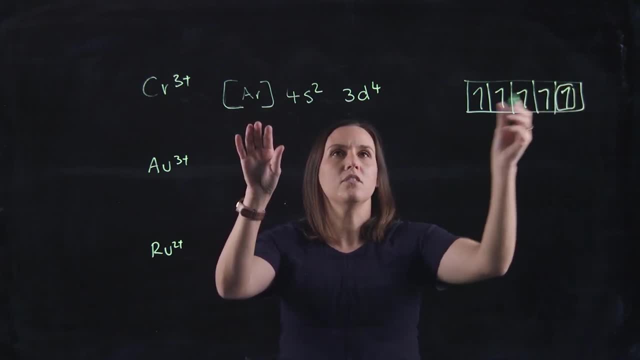 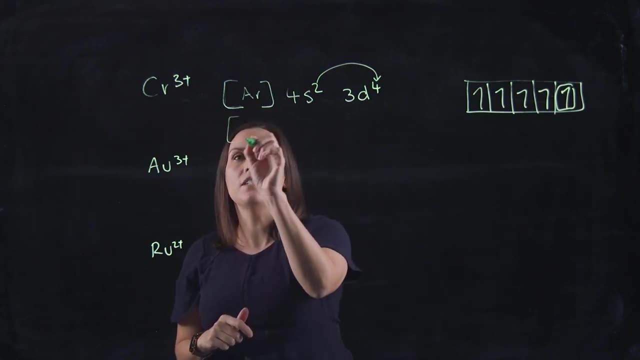 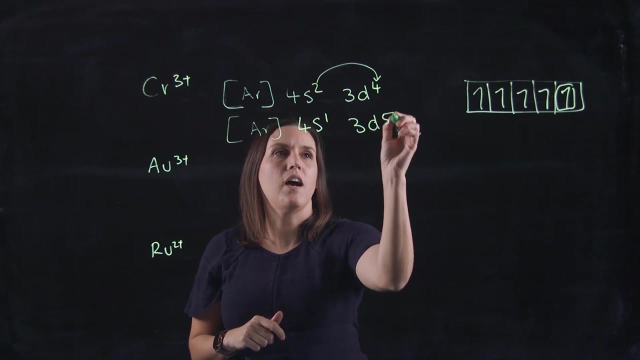 to half fill it. I would need one more extra electron. So what it does is it takes it from the s and puts it into that d block there. So the lowest energy confirmation of this would be a 4s1 and a 3d5.. So it just needs to promote one electron up from that s and put it into the d. 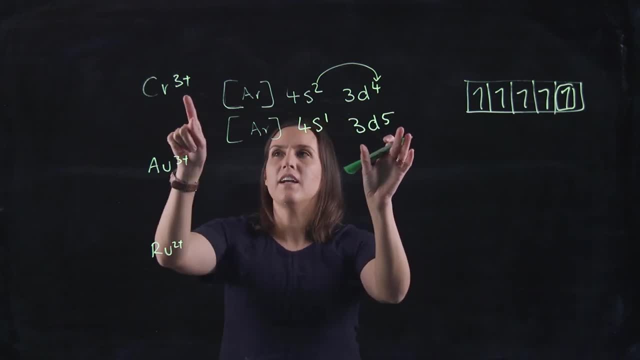 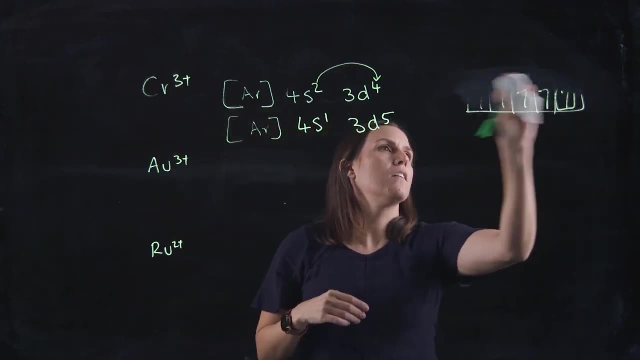 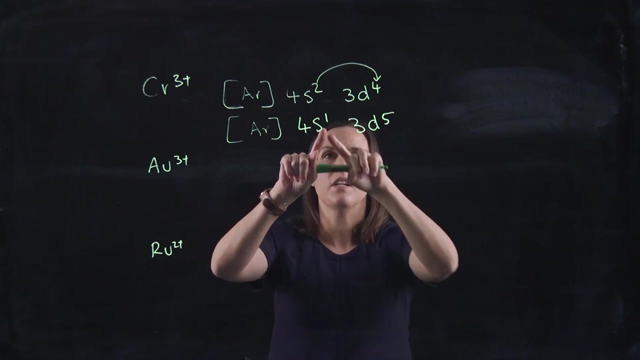 So for this one here, this is for our ground state cr. So now we've got this 3 plus here, So just make some room there. So when we have 3 plus, we're going to take three electrons. So we're going to take it from the lowest energy, which is the the 4s1, and then we're going to 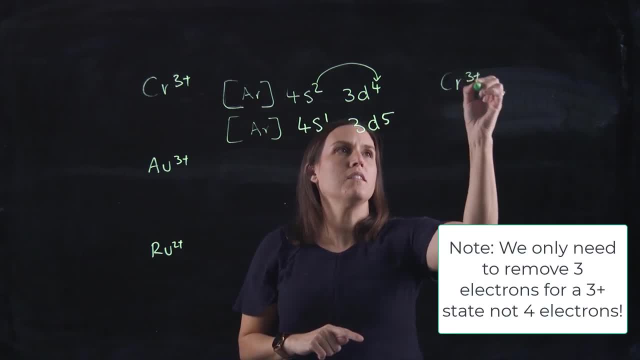 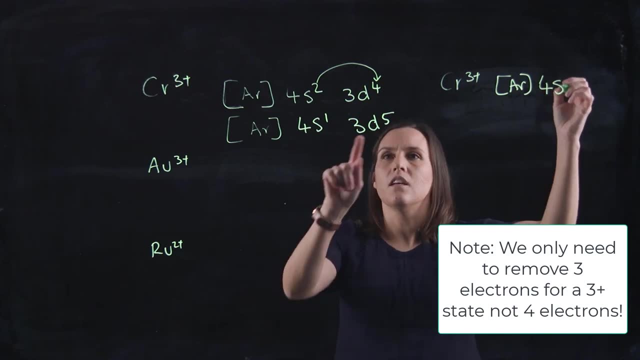 take three from that d, So the cr3 plus would be ar 4s3d. Now we're going to take those three electrons from the d, So it will come down to 3 d2, and we're going to take one from this one here, So 4s0.. So remember, we want to take from. 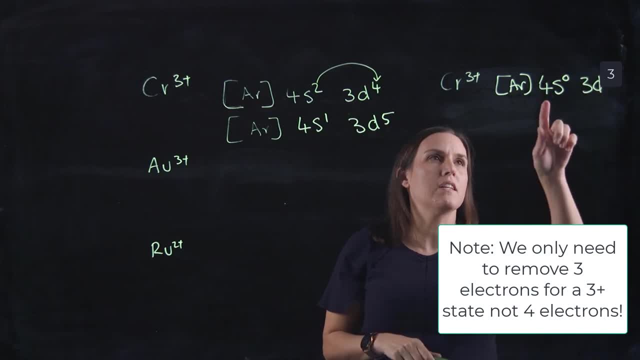 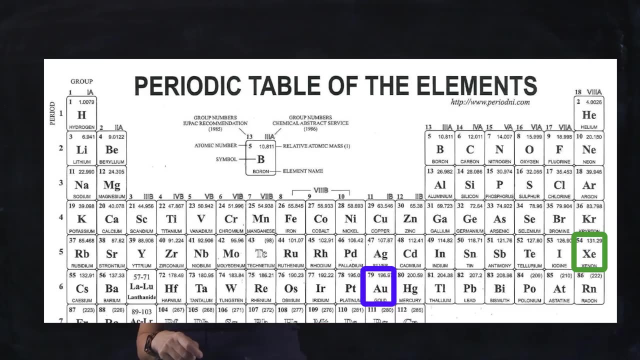 the s before we take from the d, So it's 4s0, 3d2.. So looking at gold here, so just this is just looking at cr here, Okay, so just looking at gold. So we've got xe. and then what we have after that is we have. 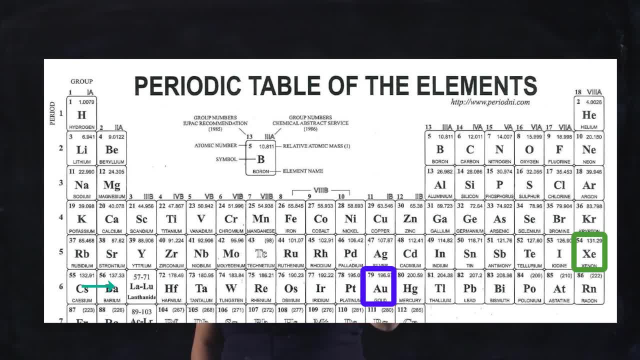 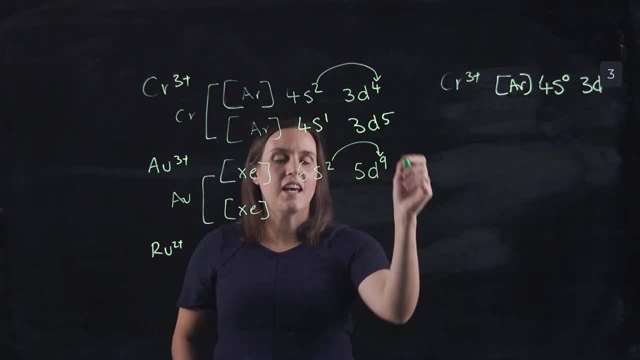 6s2- 5d, 9.. So again, we can promote one up to get to 10 there, So the lowest ground state. Okay. so taking that down, we've got 6s1- 5d10.. So we've promoted up that electron from the. 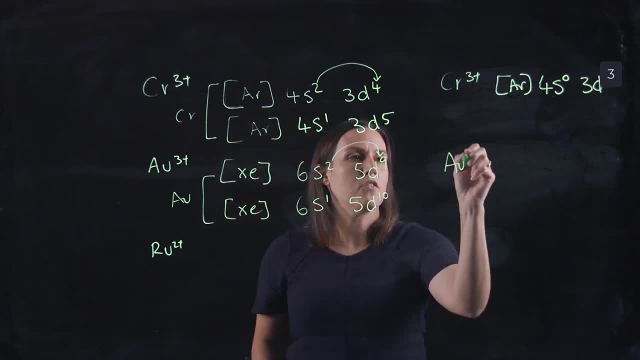 s to completely fill the d. So when we go au3 plus we're going to be taking three electrons to get that 3 plus charge. So we'll take the s and then we'll take two from that d block, So it'll be. 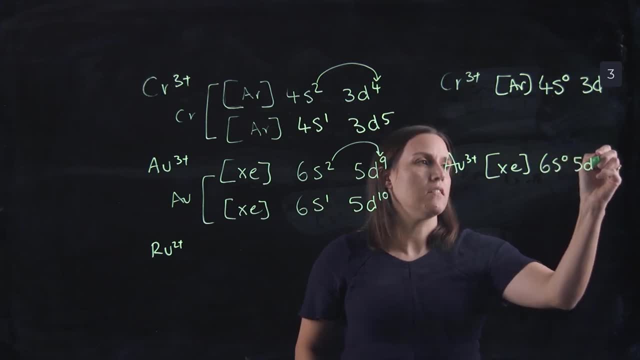 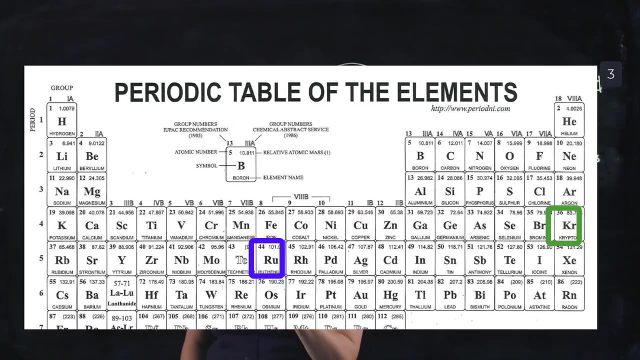 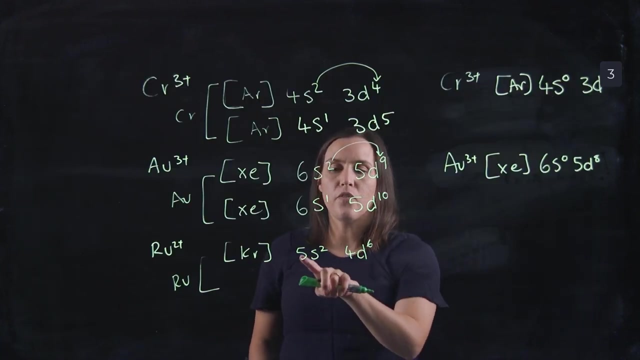 6s0- 5d10.. So now we're looking at Ru, so we've got krypton and then after that we've got 5s2- 4d6.. So looking at this one here, we've got 5s2- 4d6.. 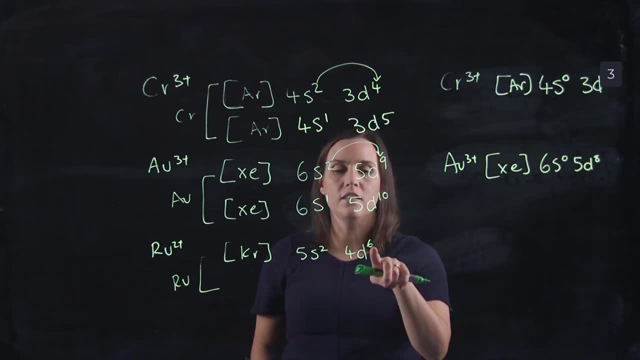 If we promote up one or two, we're not going to reach 10 because- remember our two numbers- we're going for a 5, which will give us a half field, or 10, which would give us a full d. So we won't get either of those by promoting one or two electrons. so that would be the 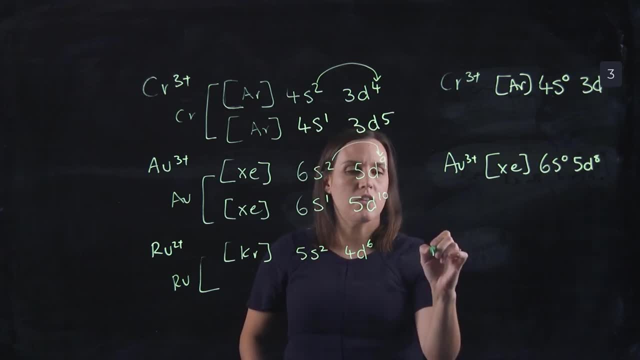 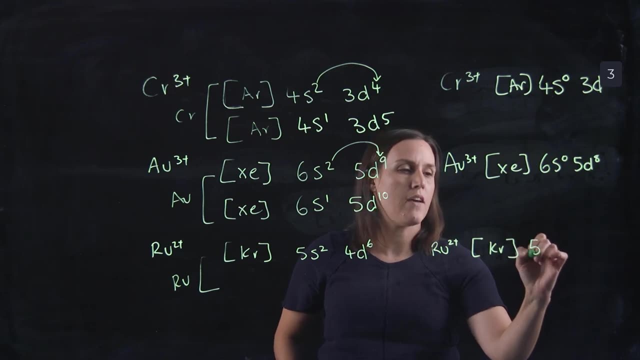 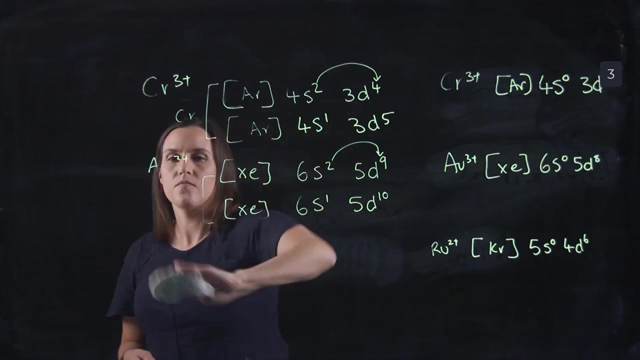 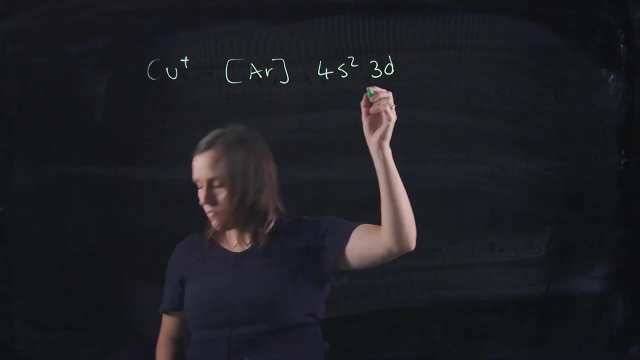 just the standard Ru. So then Ru2 plus would be taking those two away, So it would be 5s0- 4d6.. So let's have a go at some more. So, looking at copper, we end up with argon 4s2- 3d9. 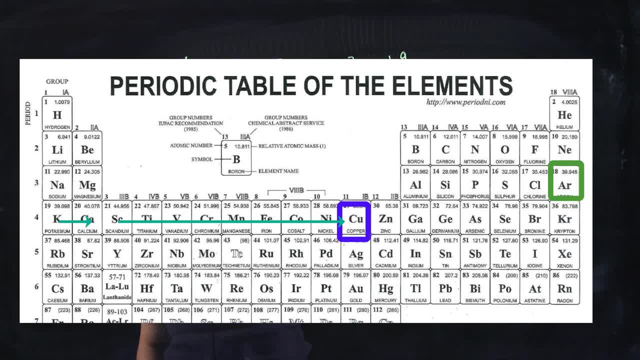 So, therefore, our So, looking at copper, we end up with argon 4s2, 3d9.. So therefore, our So, therefore, our So, therefore our plain copper would become argon, and then we would promote one of those up to get to 10.. 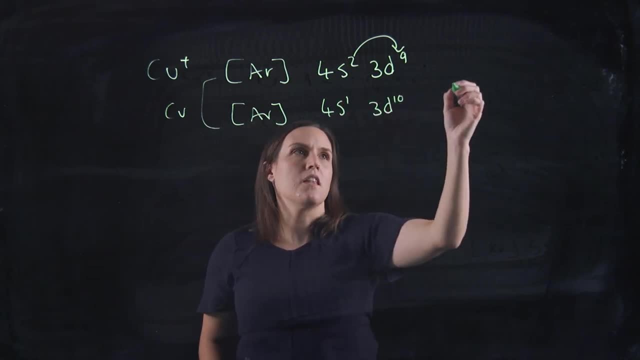 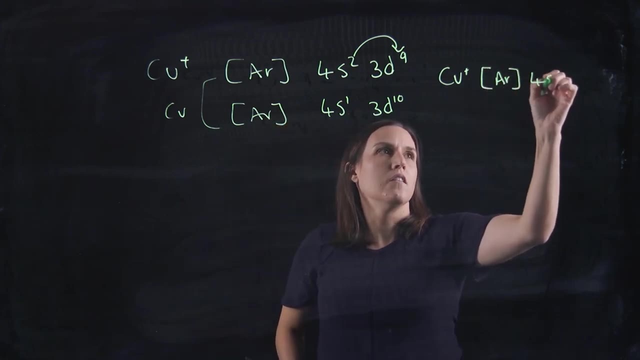 So 4s1, 3d10.. So therefore, our copper plus would be argon 4s3d. Now it's going to take this one here to get the plus, so that'll be 0 and the d would be 10.. 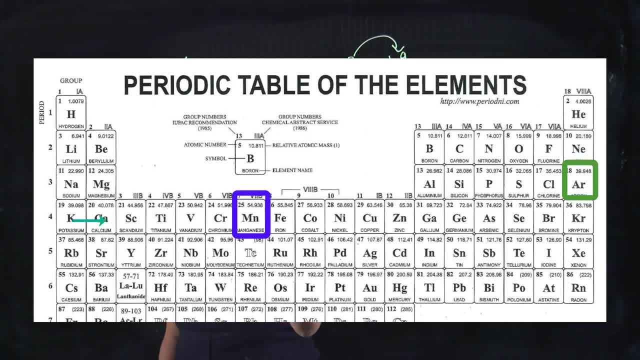 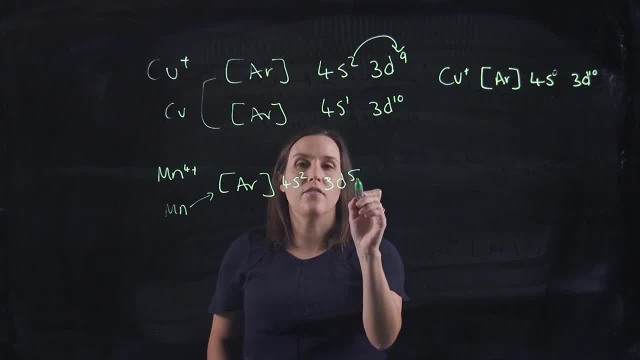 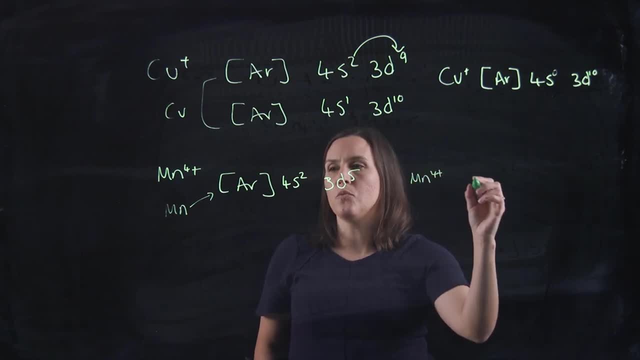 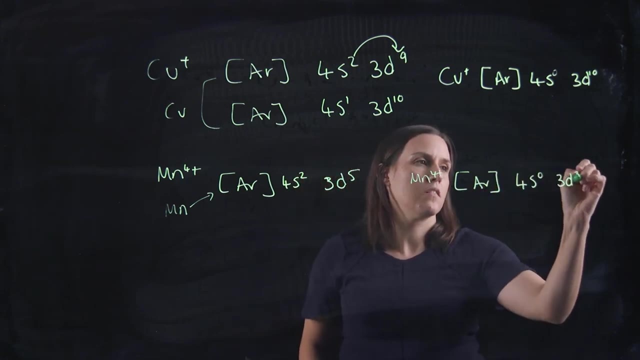 So the next one's Mn. So looking up Mn, we get argon 4s2, 3d5.. So we've got a 4 plus here. So Mn4 plus would be argon. So remember taking from the s first.